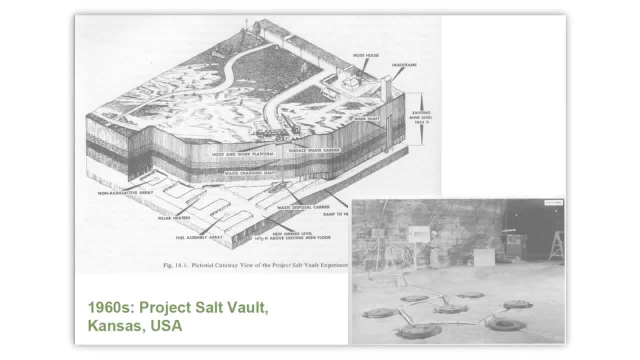 Repository In the early 1970s, an abandoned salt mine in Lyons, Kansas, is become only long term geologic repository for nuclear waste in the United States. Repository received its first waste shipment in 1999.. Since then, more than 90,000 cubic meters have come to rest here from around the US. 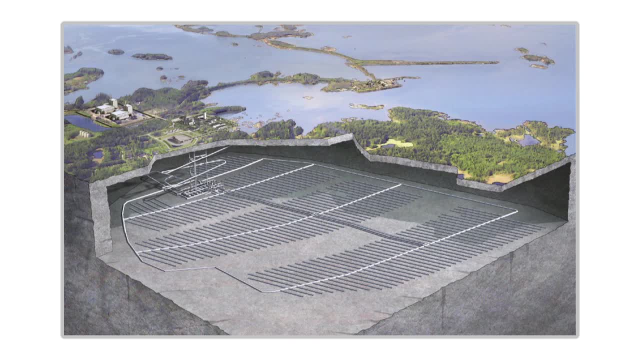 Today. example is Swedish Repository. Nuclear power companies in Sweden jointly established the Swedish Nuclear Fuel and Waste Management Company, SKB, in the 1970s. SKB's assignment is to manage and dispose of all radioactive waste from Swedish nuclear power plants. 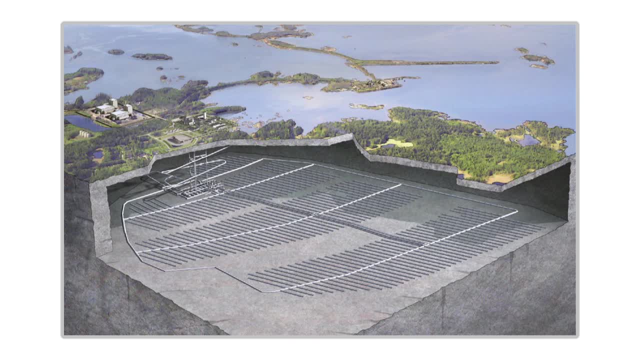 SKB is responsible for a system of facilities used to handle all waste from the Swedish nuclear power plants. These facilities include a central interim storage facility for spent nuclear fuel near Oskarshamn And a final repository for short-lived radioactive waste in Forsmark. Transport is by sea Using the vessel MS Sigrid. 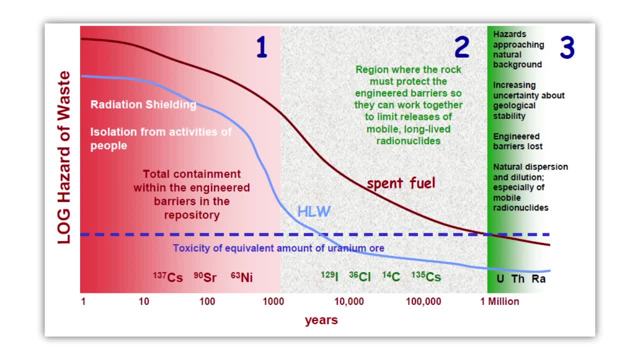 Almost any material can act as a shield from gamma or X-rays if used in sufficient amounts. Different types of ionizing radiation interact in different ways with shielding material. The effectiveness of shielding is dependent on the stopping power of radiation particles, which varies with the type and energy of radiation and the shielding material used. 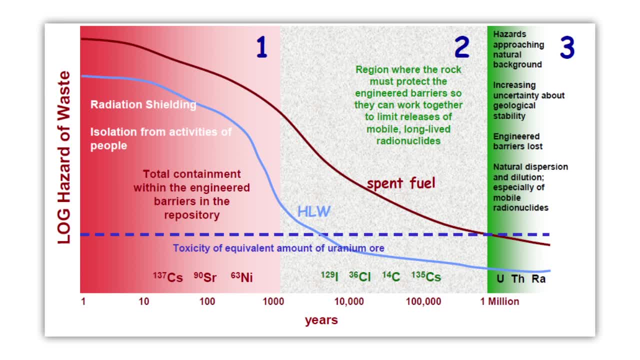 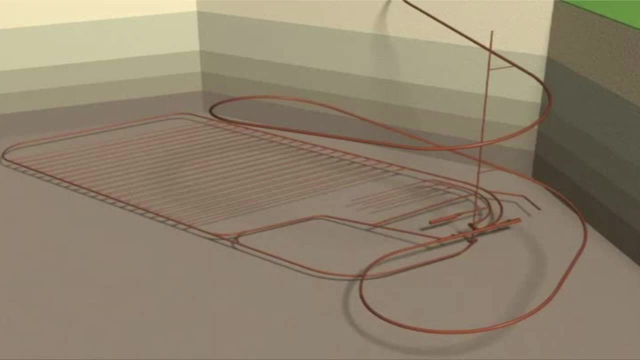 Shielding reduces the intensity of radiation depending on the thickness. This is an exponential relationship with gradually diminishing effect as equal slices of shielding material are added. In this 3-D animation we will see how radioactive waste is: delivery and store in repository. This is example of high level radioactive waste, but it can be used for all types of radioactive waste. 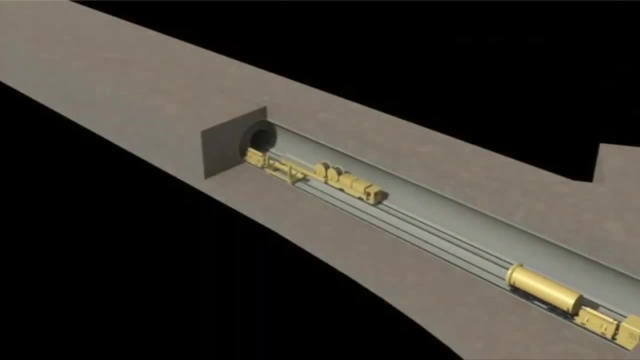 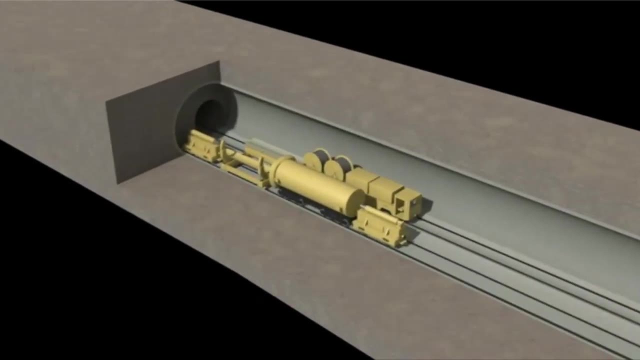 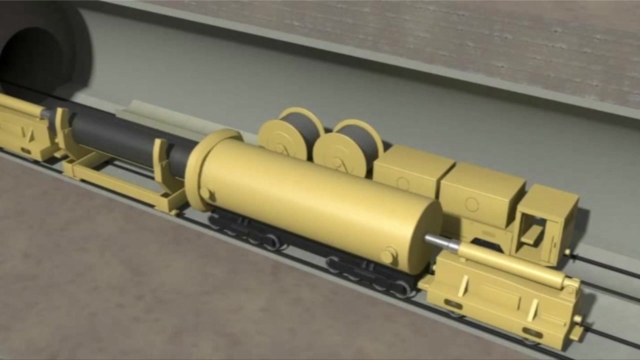 Radioactive waste is stored in dry cask cylinder made from steel. Cask are transported from above ground to the deep repository. Deep repository must be made with quality of the raw material, The rock mass, especially its fracturing homogeneity and the strength of the overburden.